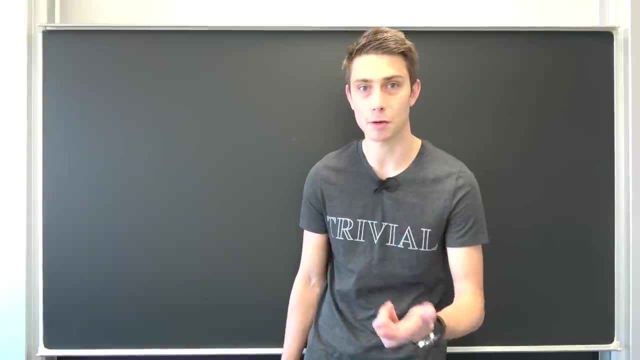 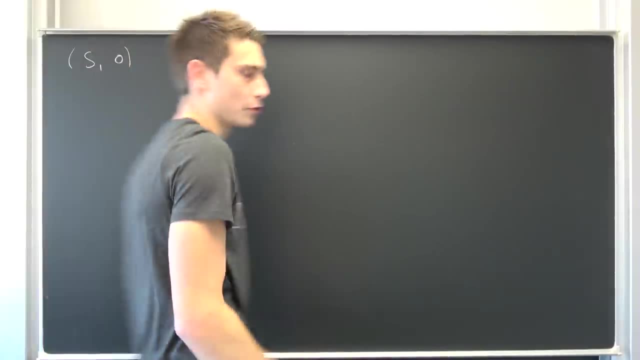 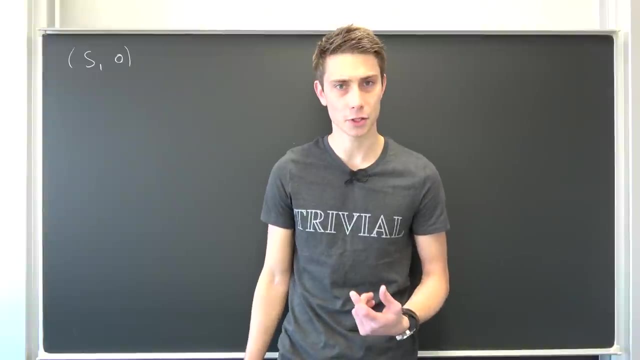 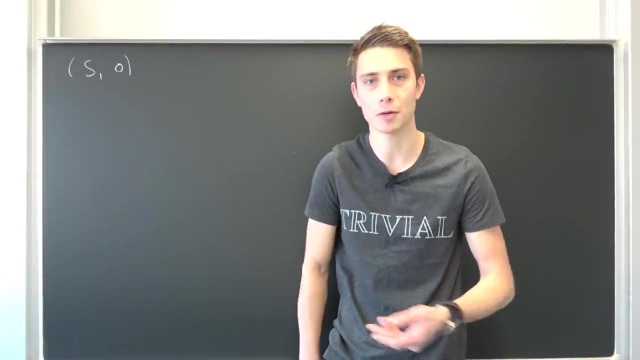 Well, suppose we have a pair being a magma, meaning it's closed under some certain operation, for example circle. So let's suppose we have some S together with a binary operation forming a magma. If this magma right here is associative, then we are going to refer to this pair right here as a semi-group. What's associativity? You might have heard of it before. You should. when working with the real numbers, natural numbers. 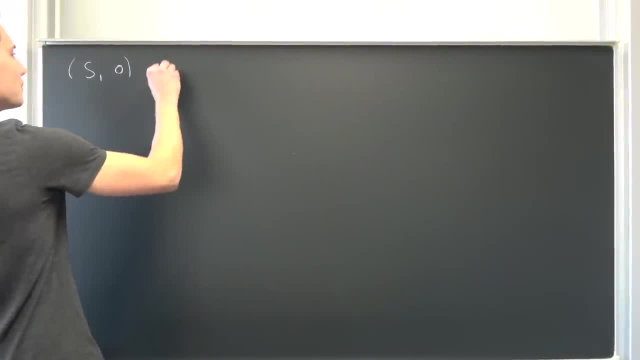 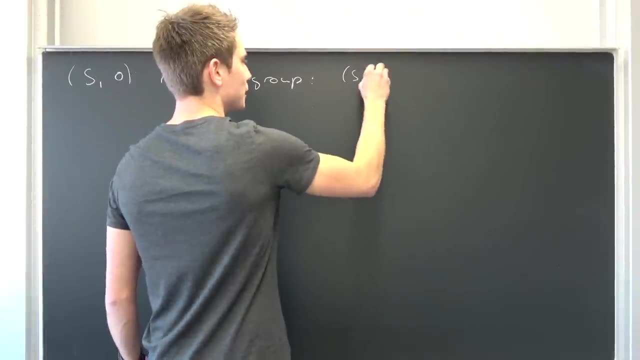 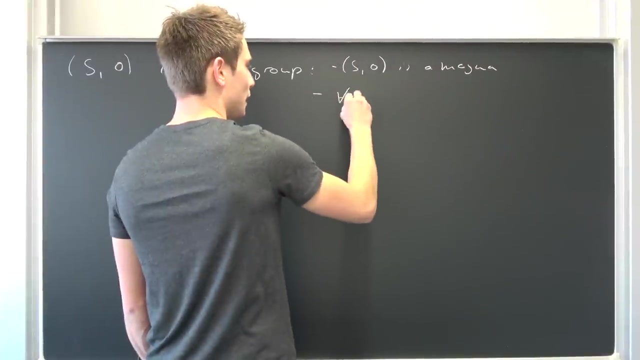 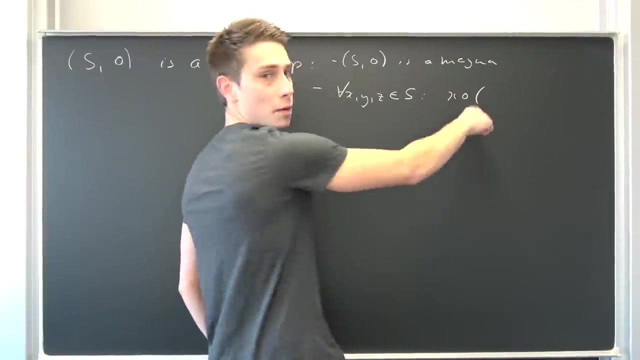 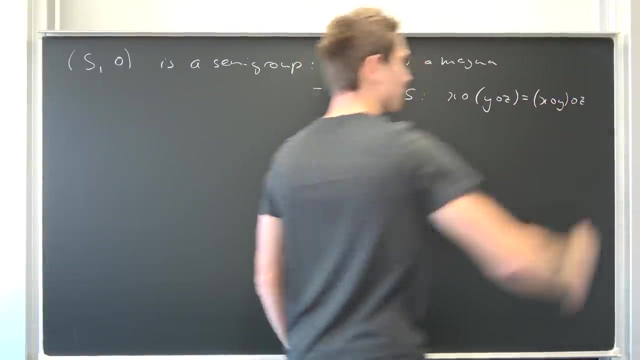 You are using it all the damn time. So associativity, So this is a semi-group. If this pair is a magma and associativity is defined, if we have for all x, y, c or z out of S, it holds that x in composition with parentheses y in composition with z is the same as parentheses x in composition with y composition with z. 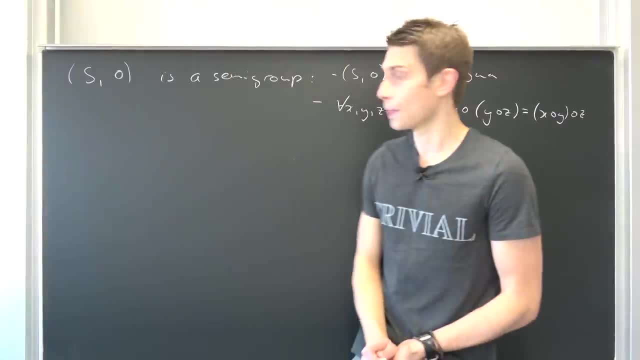 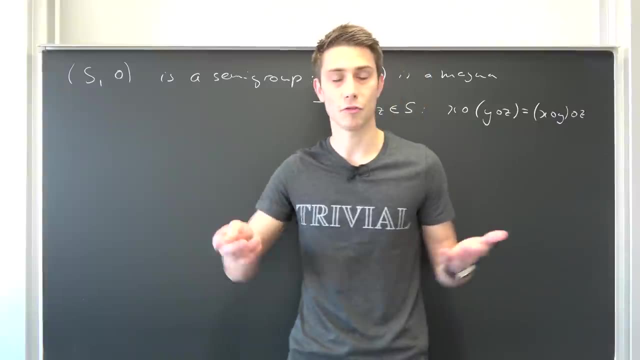 This right here is called a semi-group, This is called associative property, And well, if this holds, then we are going to refer to this as a semi-group. Also, if this semi-group has only a finite number of elements, this is going to be a finite semi-group. 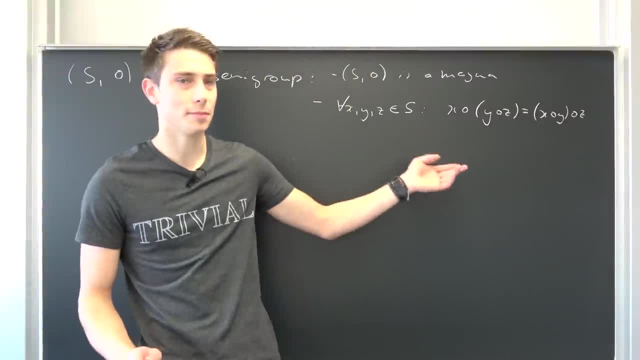 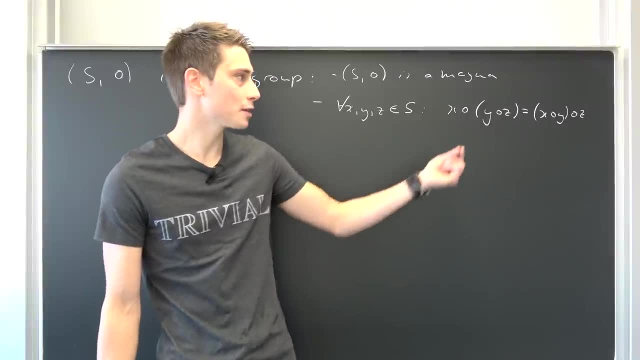 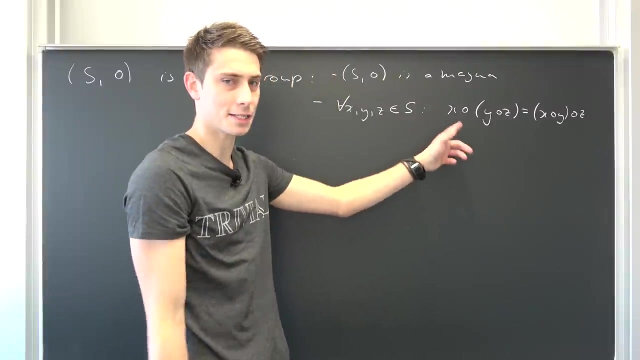 It does make sense. So associativity basically means that the order of carrying out the operation is not relevant at the moment, but it's relevant in which order we are going to carry out the operation, meaning on our operands. So x times y is not relevant. 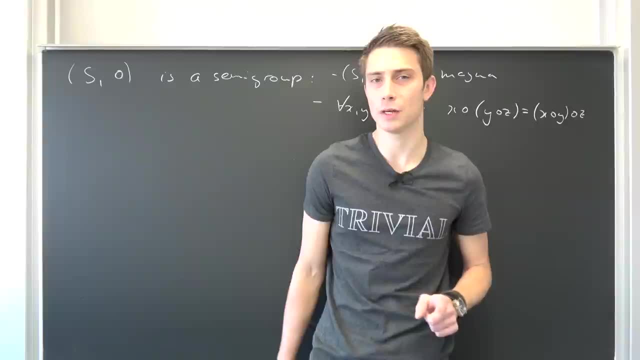 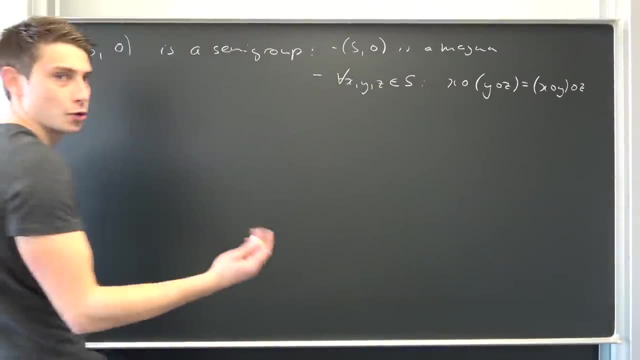 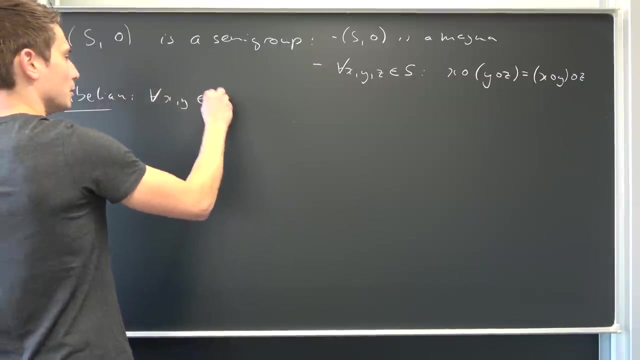 It's not the same as y times x, But if it would be the same, then we would refer to this right here as being abelian. So what's an abelian algebraic structure? Well, abelian just means if for all x and y element of S it holds that x in composition with y is the same as y in composition with x. 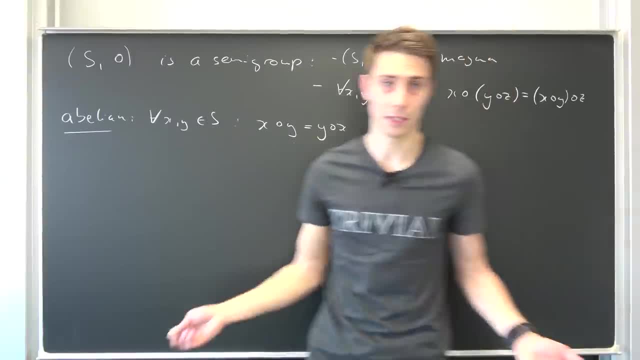 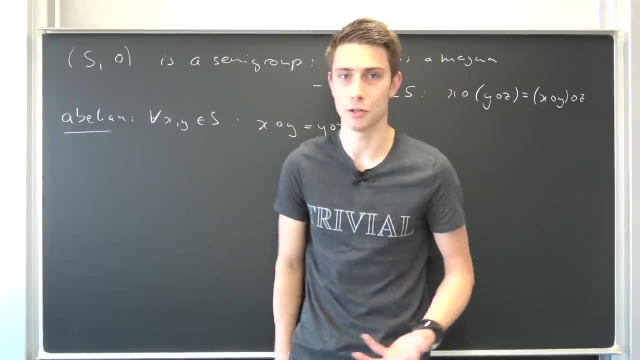 And we can also have magmas which are abelian. Most of the time, people are going to say, well, that's not true. That's not true. Most of the time, people are going to refer to abelian as just commutative. 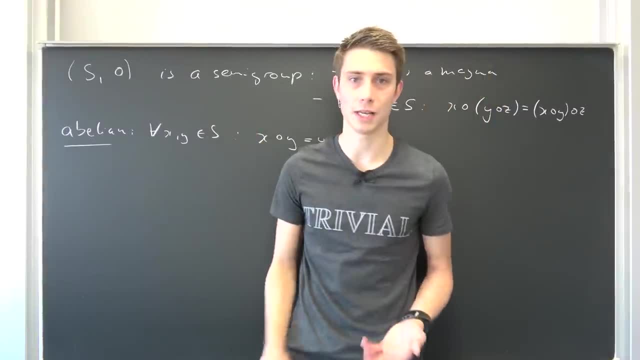 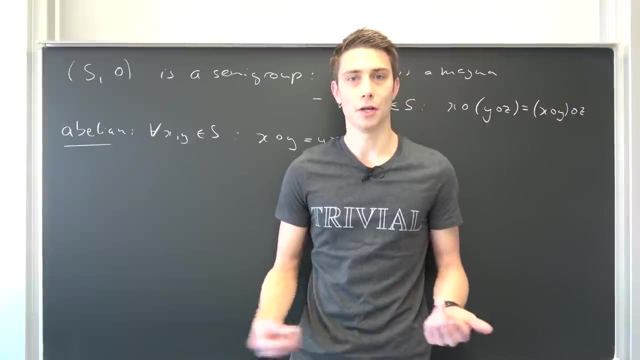 So you can also refer to this as a commutative semi-group. then OK, with this out of the way. we are going to prove today that the natural numbers under addition form an abelian semi-group, meaning we have already shown that the natural numbers under addition form a magma. 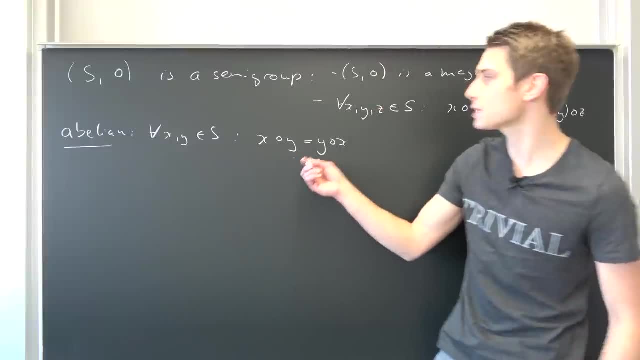 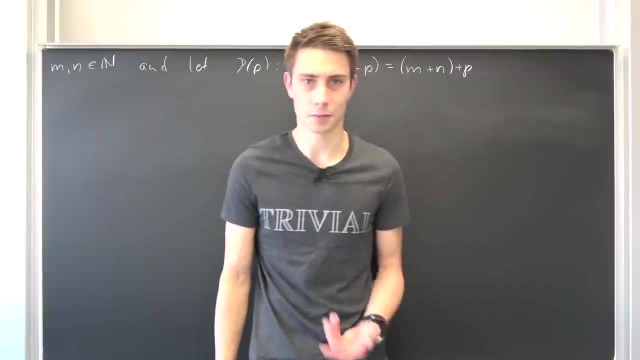 So all that's left to show is that this property holds for all natural numbers and that this property holds for all natural numbers. We're going to do this in the next part, So, as always, we are going to make use of the principle of mathematic induction. 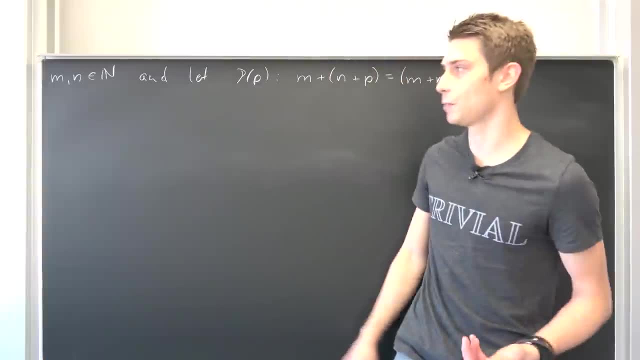 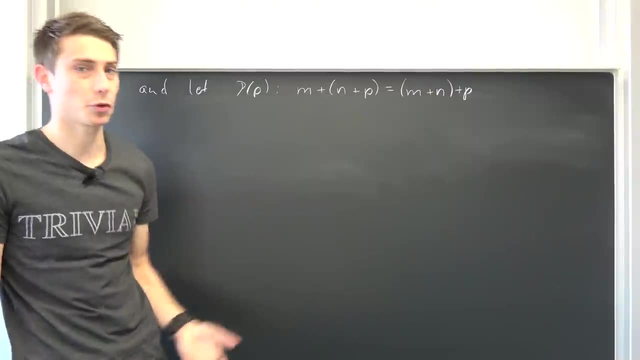 And this, right here, is our proposition. We are going to take some n and m fixed by the arbitrary natural numbers, And this is our proposition, p of p, And we want this to hold for all natural numbers. So that's what we are going to prove now. 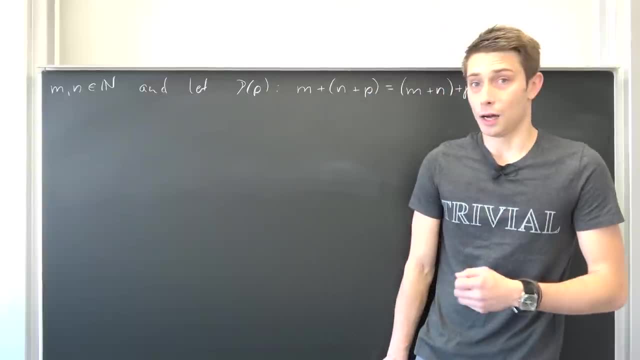 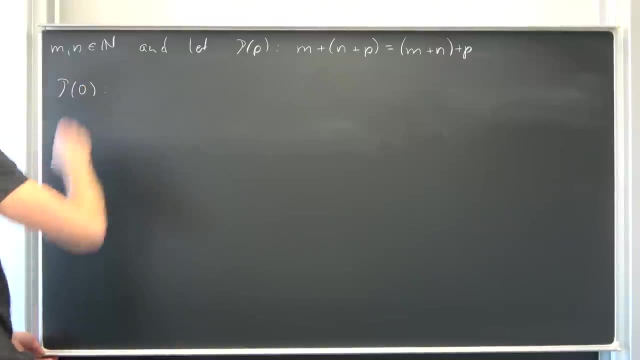 So p is our dependent variable. you could say, OK, so let's go ahead and get started with the base step. p of 0.. So p of 0, what is that exactly? Well, we are going to plug 0 into here. 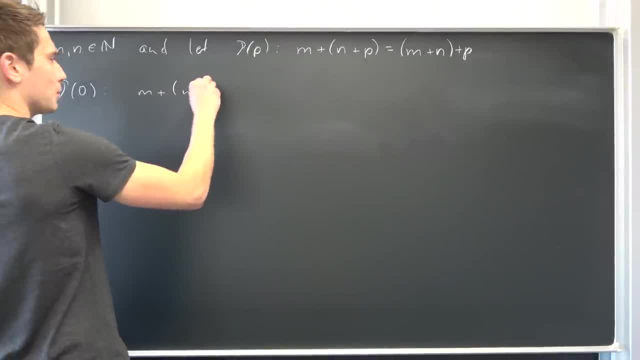 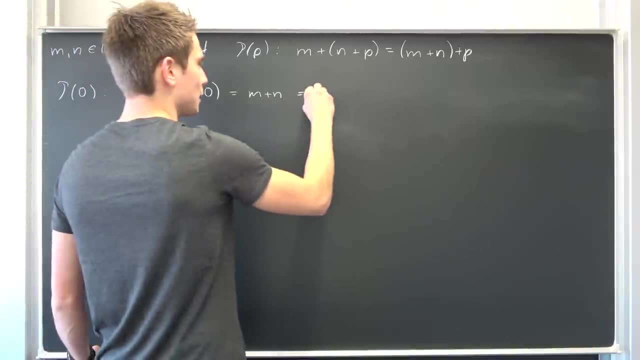 We're going to plug 0 into here, So we have m plus n plus 0.. Well, this is nothing but by the first part of addition, m plus n. But this is nothing but m plus n, in parentheses, plus 0.. 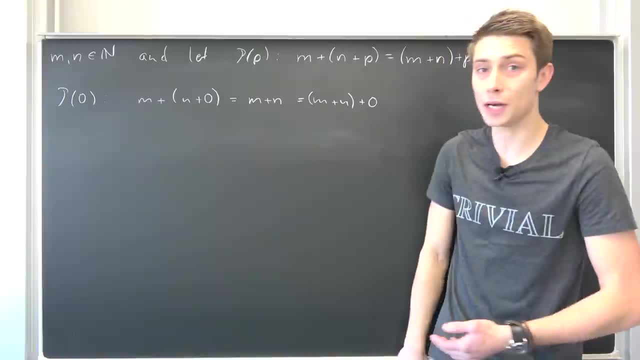 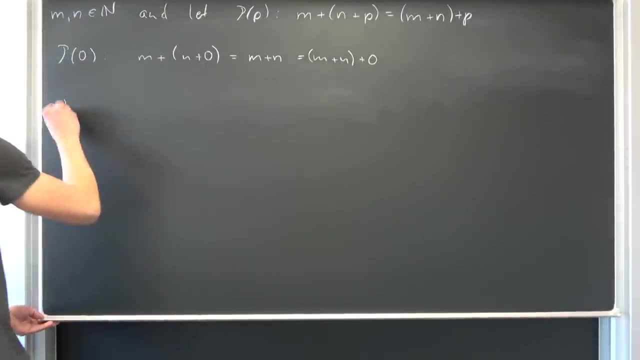 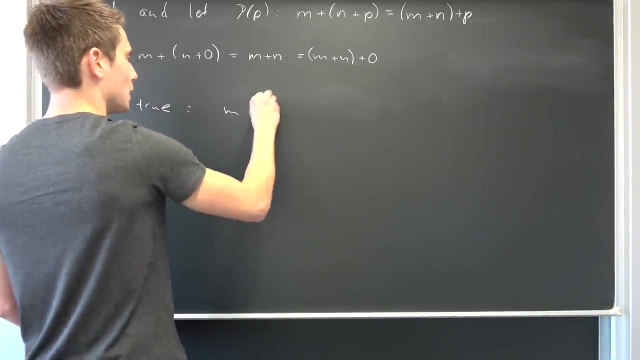 OK, you see, this has been the base step, really quite easy. And now we are going to assume that, well, our proposition is true for some random arbitrary k out of natural numbers. So p of k is true, Meaning. Well, this is nothing but m plus n plus k equals to m plus n plus k. 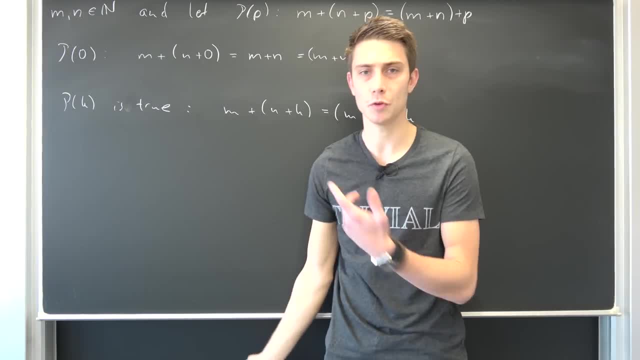 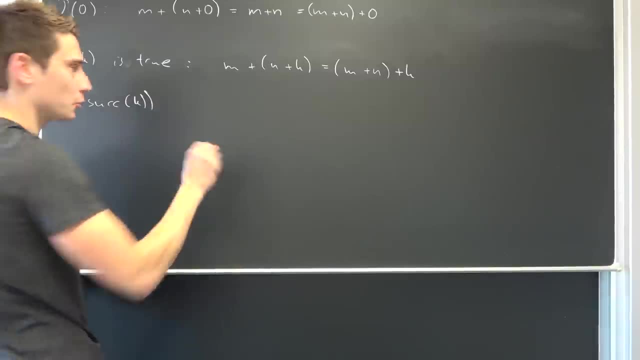 And now we want to show if this ensures our proposition to be true for p of the successor of k. So for p of suc of k, What are we going to get? Well, this is nothing. but why not start off at this side? for example, 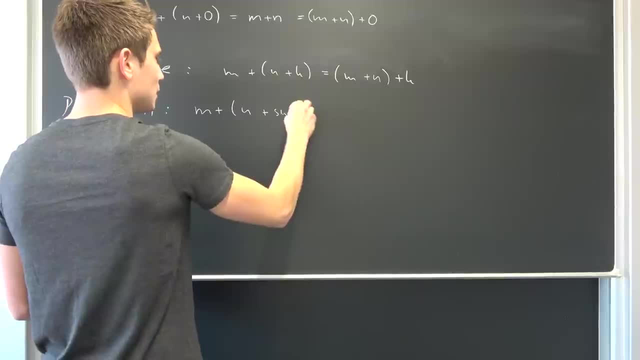 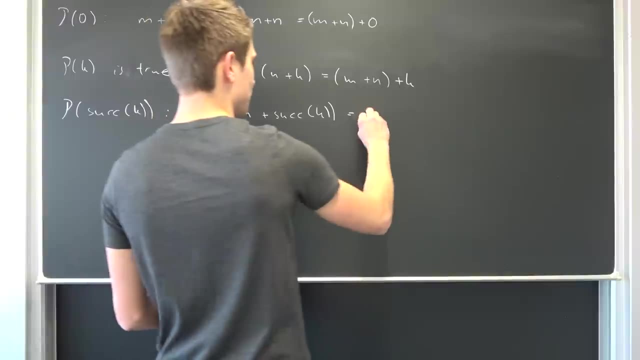 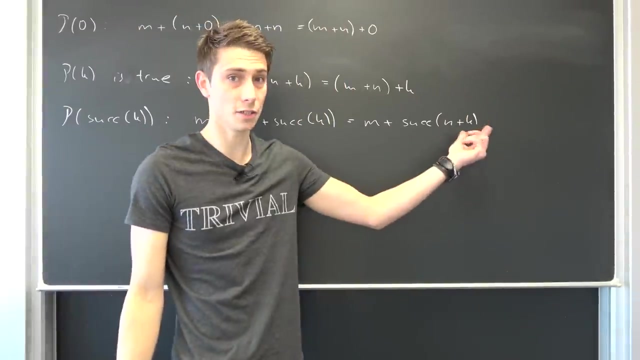 So we have m plus n plus suc of k. OK, We also know by the second part of addition that we can drag the suc to the front right here. So this is nothing but m plus suc of n plus k. But once again, this is closed under addition. 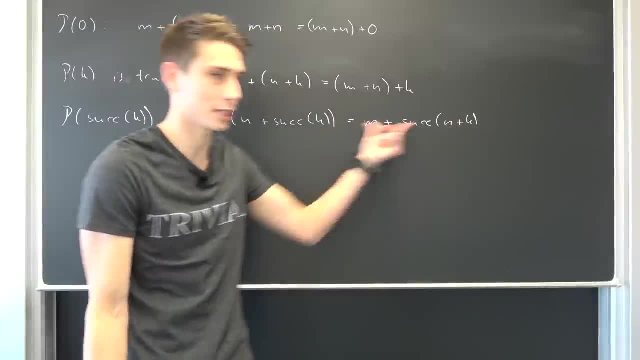 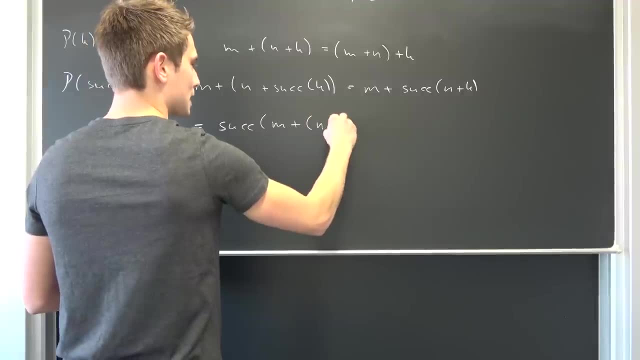 We have shown that this is a magma, So this is just an element of natural numbers, So we can just drag the suc to the front once again. So we have the successor of m plus parentheses, n plus k, And now we are going to make use of our induction hypothesis meaning by p of k. 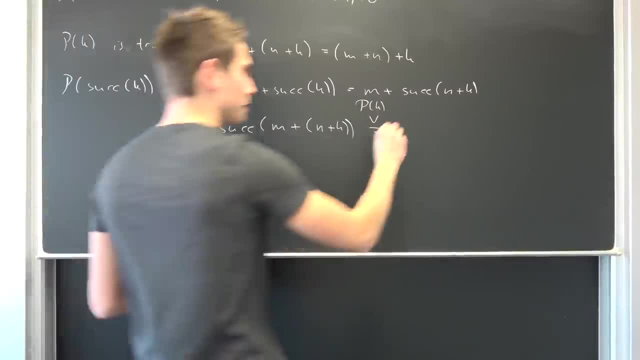 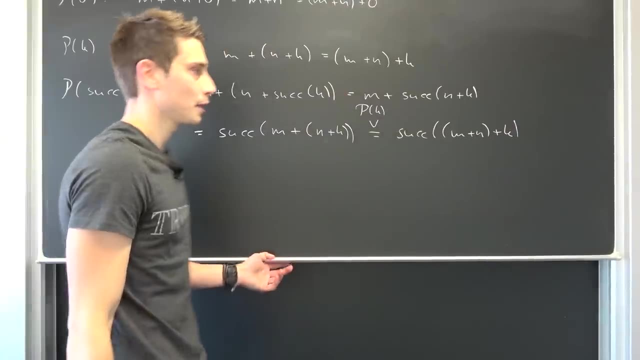 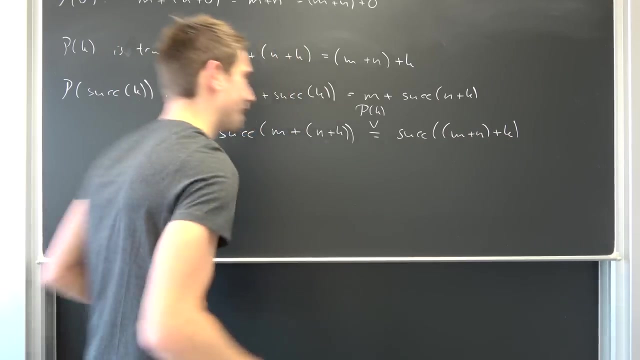 We can interchange those parentheses right here to the successor of parentheses m plus n plus k, And you see, this right here is just some natural number. So we can reverse this second rule of addition and bring the suc to this k right here. So this is just how it works. 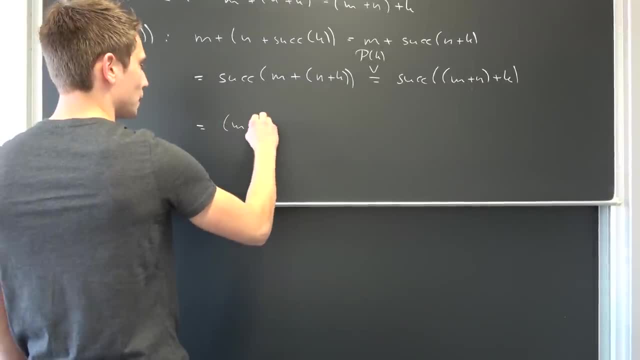 If this is a natural number, then this is going to hold. So we have m plus n plus successor of k, And then we are done. So we have shown that this right here is the successor of m plus n plus k. OK, 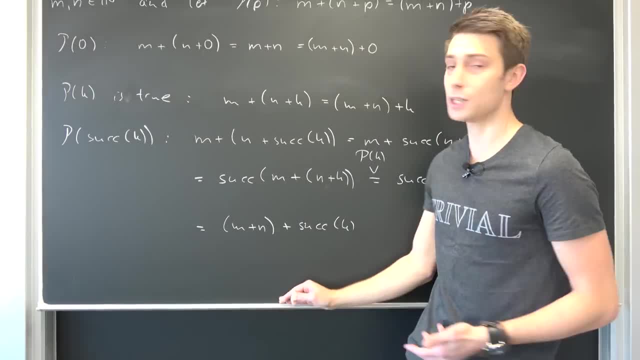 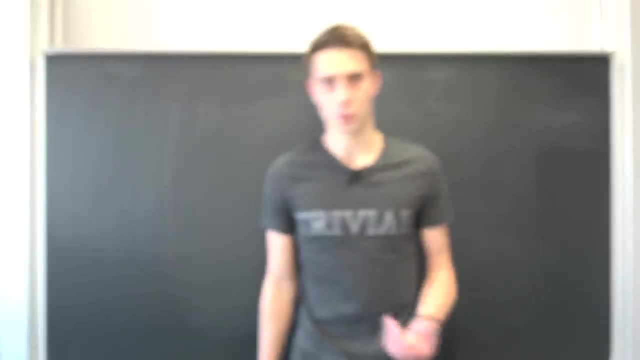 So this right here is an associative operation, meaning at the moment our natural numbers under addition form a semigroup. And now for the abelian part. So to show that this is abelian, we have to make sure that our base step would even hold. 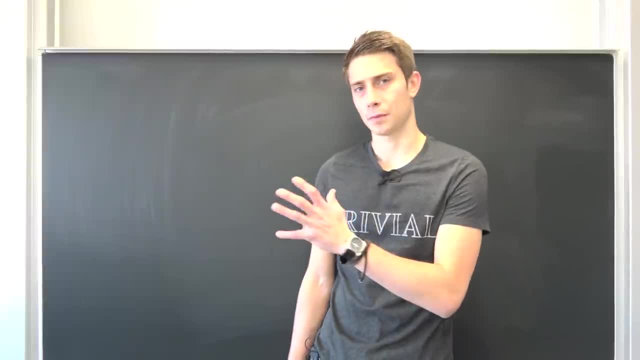 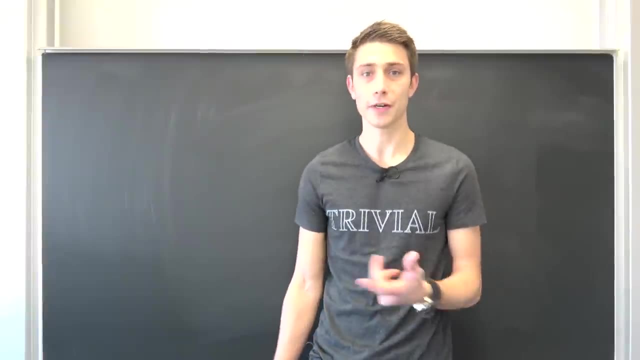 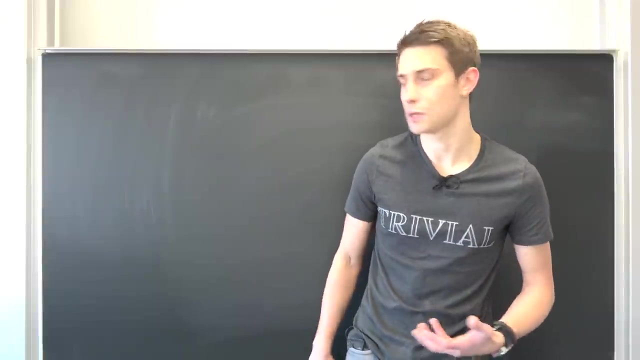 So for our base step to hold in regards to our abelian structure, we have to make sure that our zero is going to commute under addition with every other element out of natural numbers. Zero is kind of special. We have to treat it differently, sometimes in a certain different process. 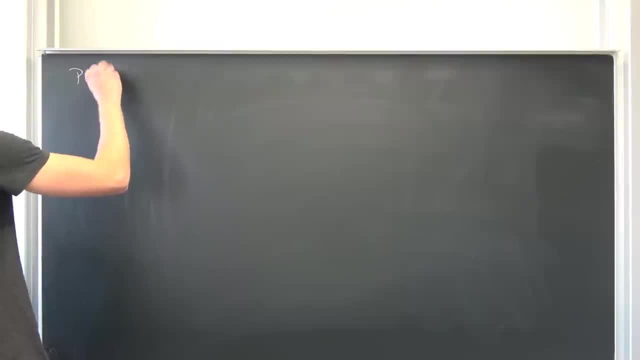 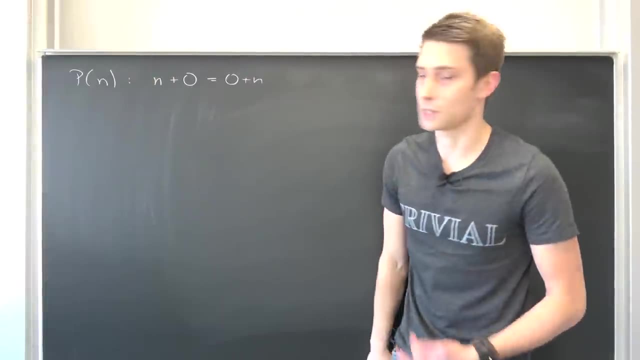 So why not show that p of, let's say n, is nothing, but n plus zero equals to zero plus n for all n out of natural numbers. So this, right here, is our proposition, and we are going to start off with the base step once again. 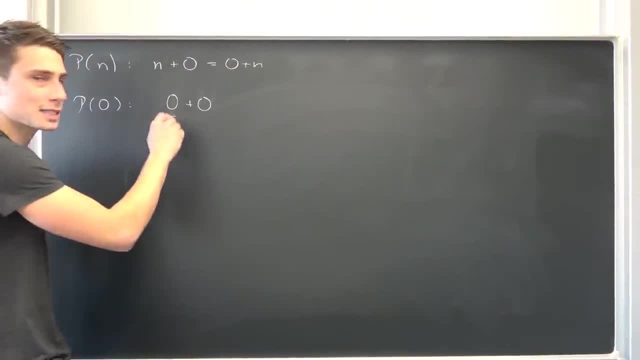 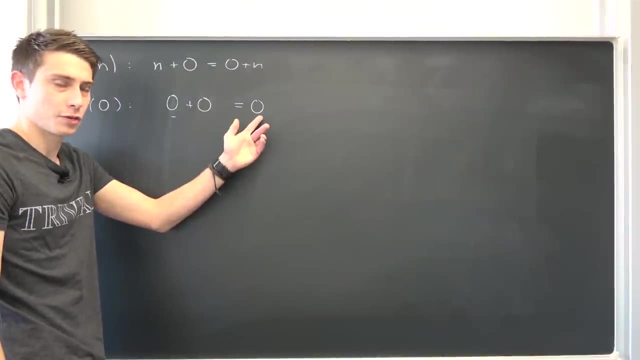 P of zero. Well, this is nothing but zero plus zero, where this is our zero that we have plugged in. But by the first rule of addition, this is nothing but zero. But we can add a zero to this by the first rule of addition and it wouldn't change anything. 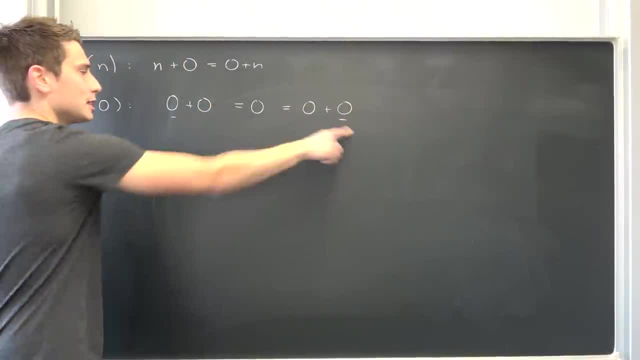 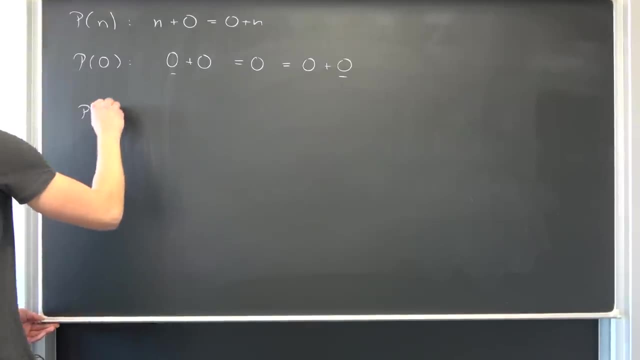 So this is zero plus a new added zero. So you see, we have shown that the base step holds And now we are going to assume that p of k is true. for some random arbitrary k out of natural numbers. It's going to be fixed. 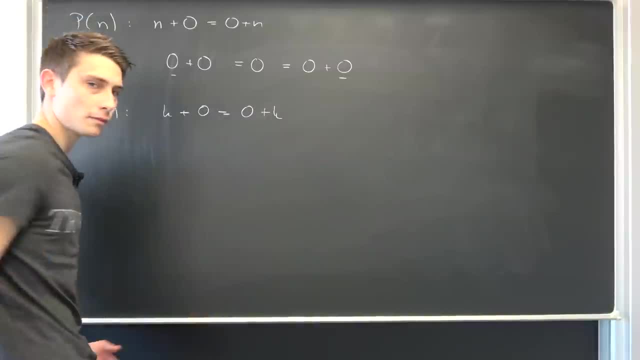 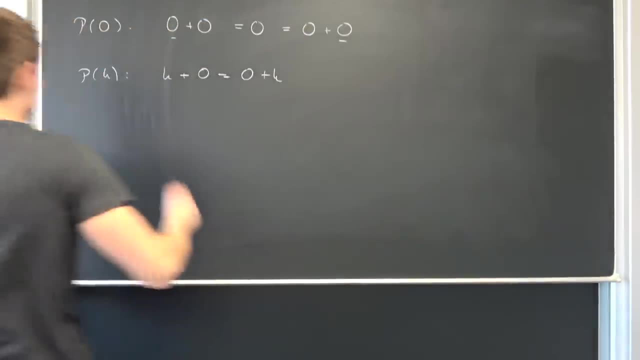 So k plus zero is nothing but zero plus k. Once again, we want to make sure that this thing right here ensures our proposition to be true for the successor of k. So let's go ahead and get started. P of suck, P of k. 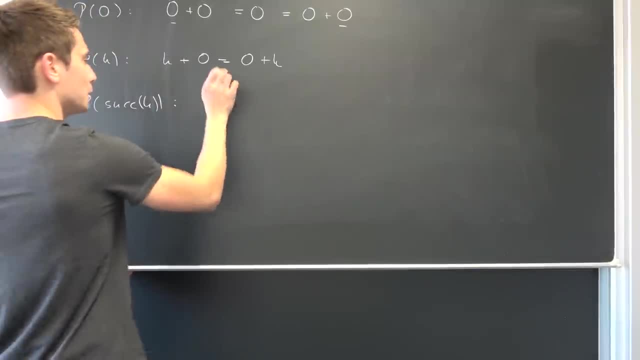 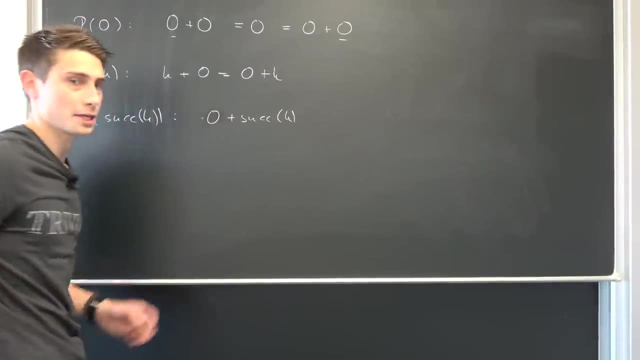 What is that exactly? Well, this is nothing, but yeah, we are going to start off from this side. it really doesn't quite matter. So we have zero plus the successor of k. Why am I starting from this side? Well, we want to make use of the rules of addition, right here. 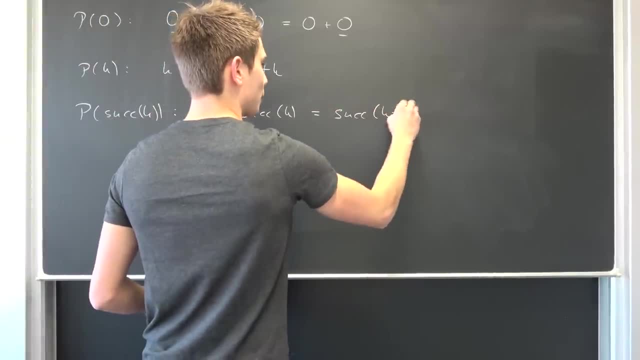 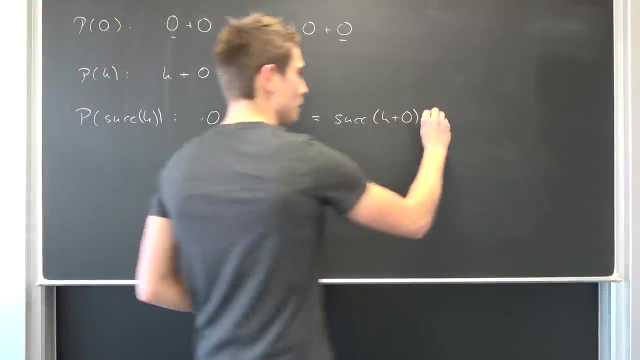 Second rule of addition: So this is nothing but the successor of k plus zero. But you see, k plus zero is just well k itself. So first rule of addition: So this is just the successor of k, But right here it wouldn't really hurt us to add a zero to this thing. 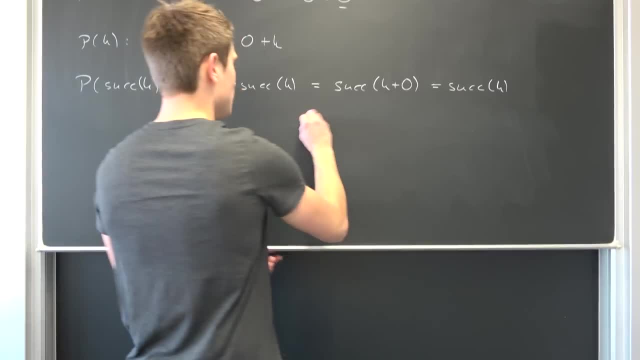 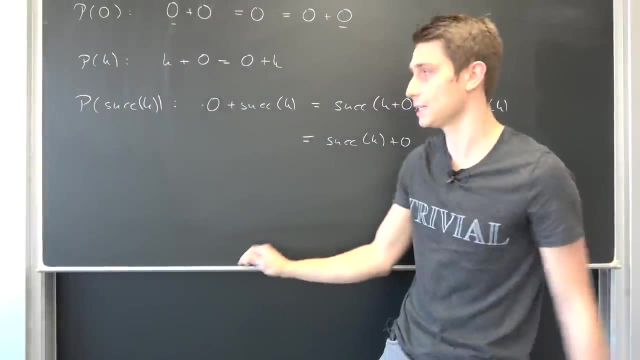 But the first rule of addition, it does work. This is just element of natural numbers. So that's the same as saying we have the successor of k plus zero. Hey, we have shown that the zero commutes with every element. here on the natural numbers, 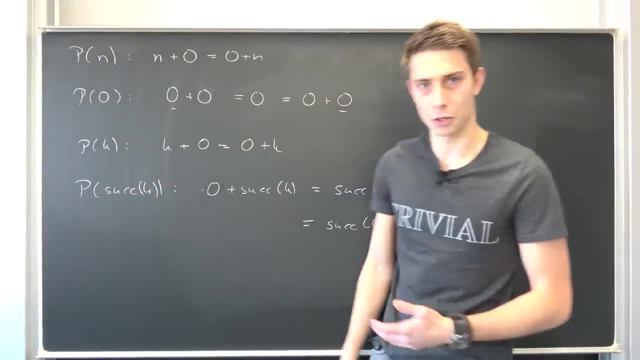 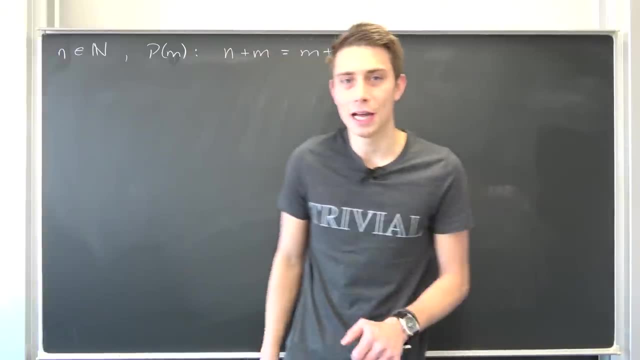 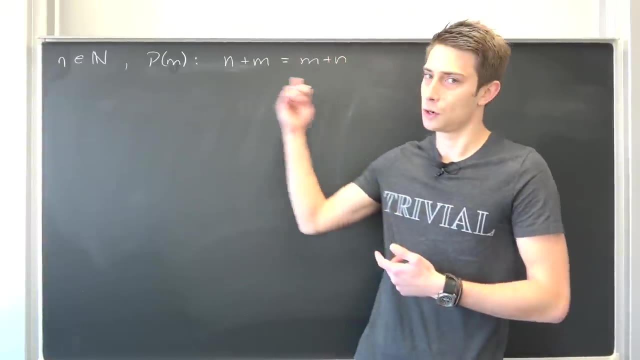 We have laid the groundwork for our big proposition that we want to show now And, yeah, we're going to go ahead. This last part is really quite fiddly, But it's doable. Okay, It's doable. We have laid all the groundworks, like associativity and commuting property of the number zero. 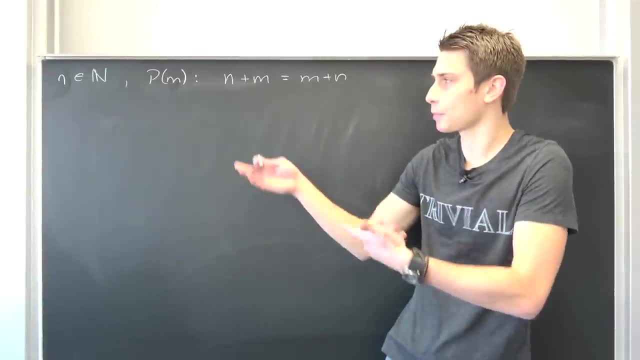 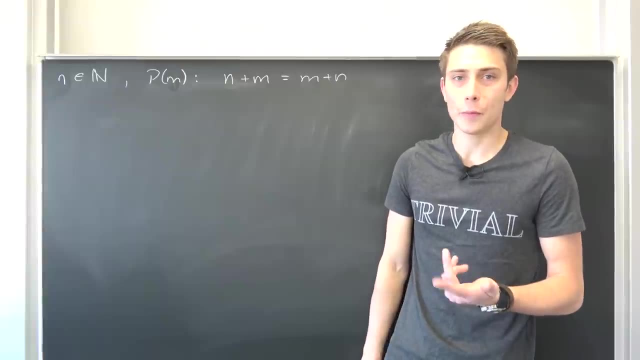 So you see our base step p of zero is well, completely clear from our previous lemma. we have just derived So that the zero commutes with everything. Now we are going to introduce some p of k once again for some random arbitrary fixed. 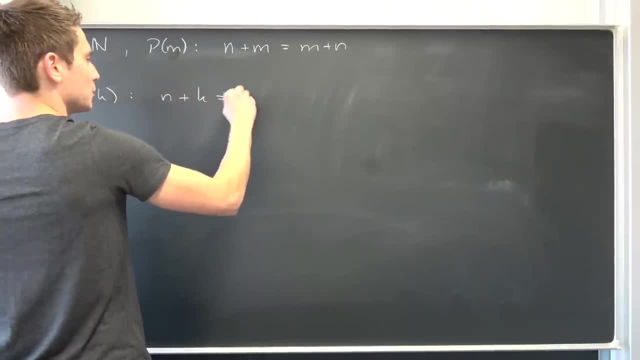 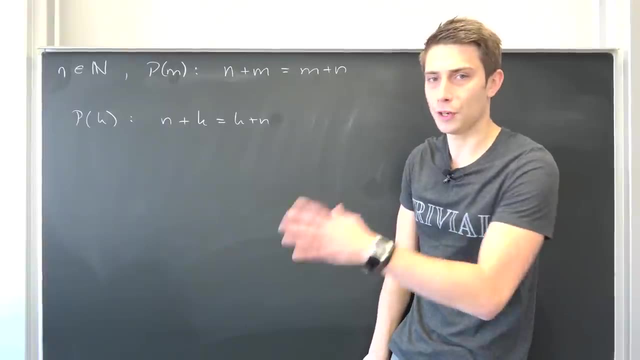 natural number k, which is nothing but n plus k, is equal to k plus n. So we have a natural number n out of natural numbers fixed, Not for all natural numbers, for some natural number n which is fixed. I'm terribly sorry. 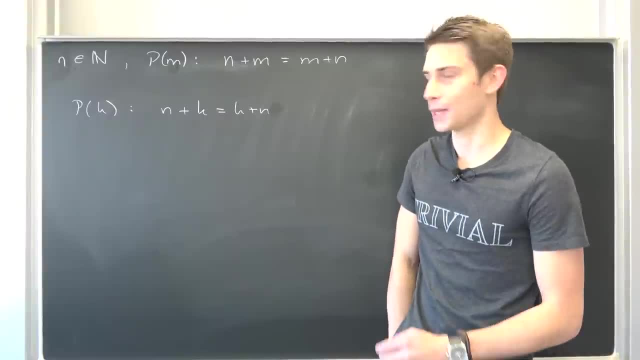 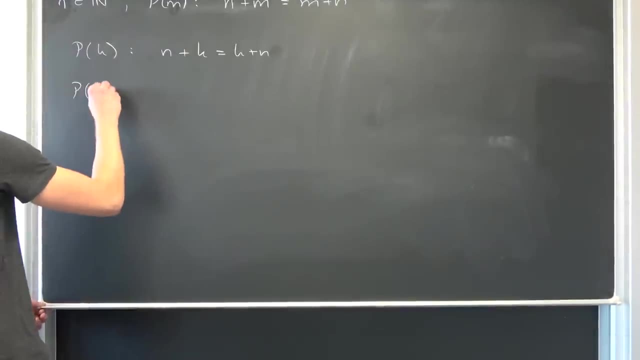 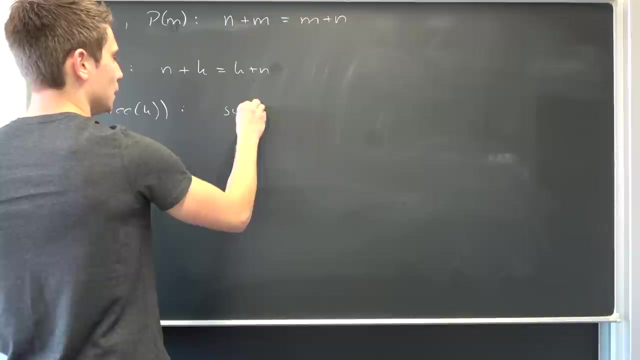 I rephrase this a little bit badly. Once again, we want to make sure that this ensures our proposition to be true for the successor of k, So p of suc of k, And we're going to start from this side. So this is nothing but well, plugging the successor of k in at first, plus n, But by 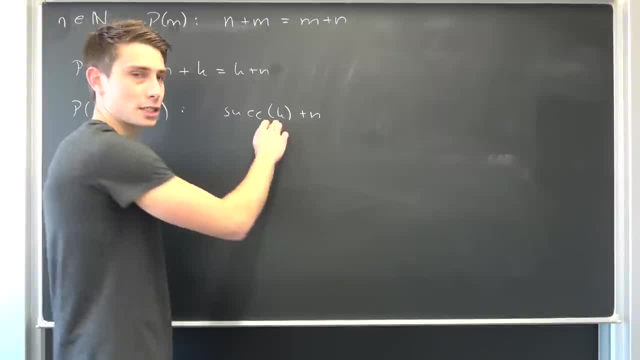 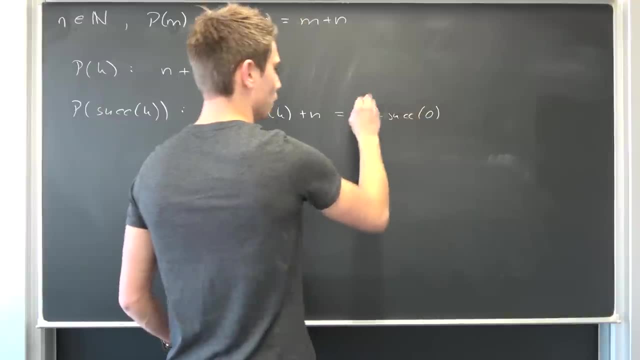 by some proposition we have introduced at the start of the series. We know that the successor of k is nothing but k plus the successor of zero. So this is nothing but k plus the successor of zero- Putting this in parenthesis because this is a number for itself. 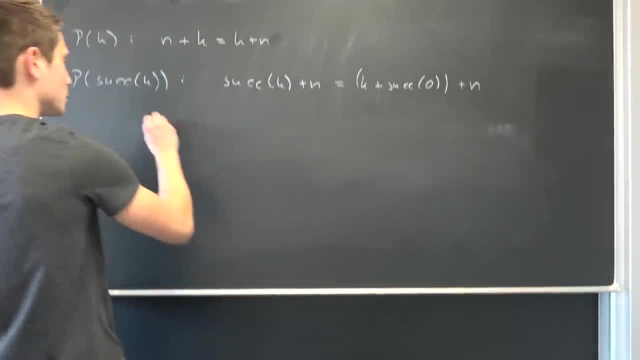 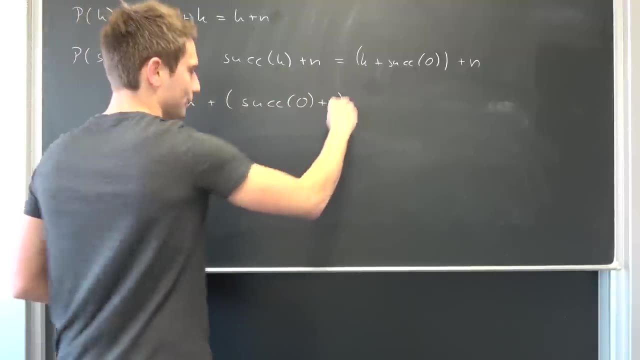 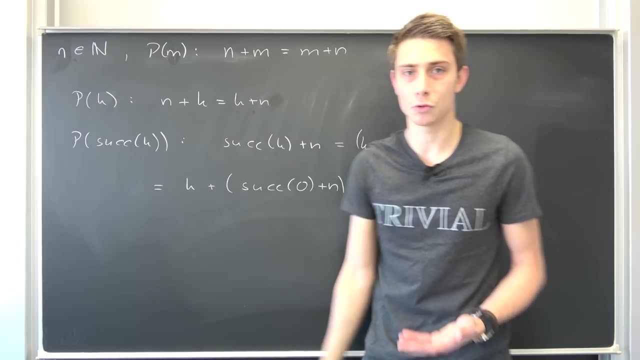 But we have introduced the associativity right now, So we can just use the associative property to turn this into k plus well, parenthesis, successor of zero plus n. Okay, So Okay. But by our proposition we know that our well, natural numbers are going to commute.